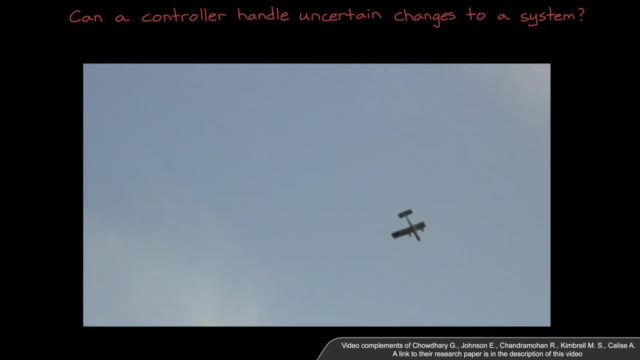 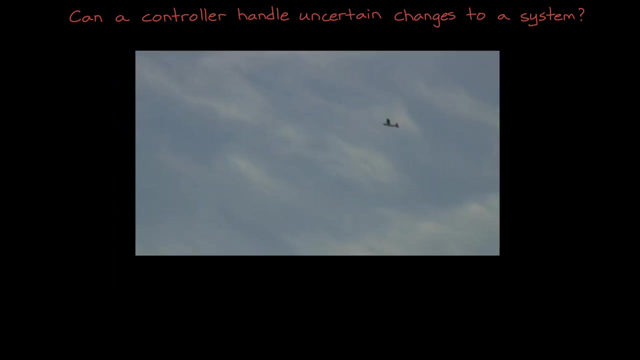 that- is that something you should have expected- and built in some kind of wing broken mode in the controller? Or can you just design a controller that's able to adjust itself to this new, unexpected situation on its own? Well, that is what adaptive controllers can do, and in this video we're going. 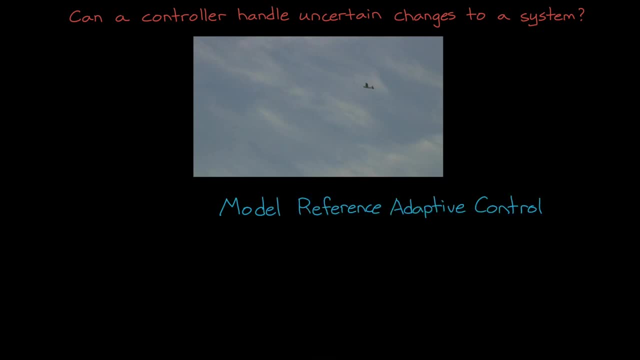 to talk about one adaptive method called model reference adaptive control, And so you know what you're getting yourself into. this is just an introduction to the topic. We're not going to go too much into the mathematics of this control law, but I do think it will be interesting and 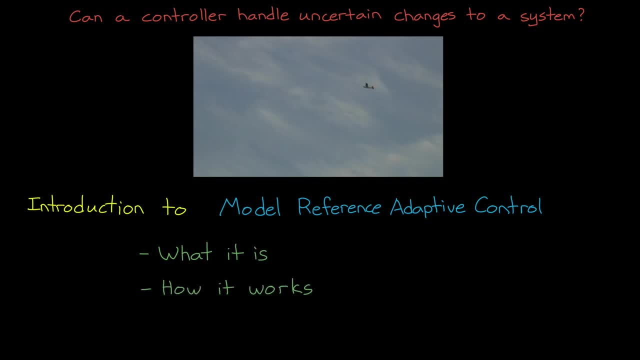 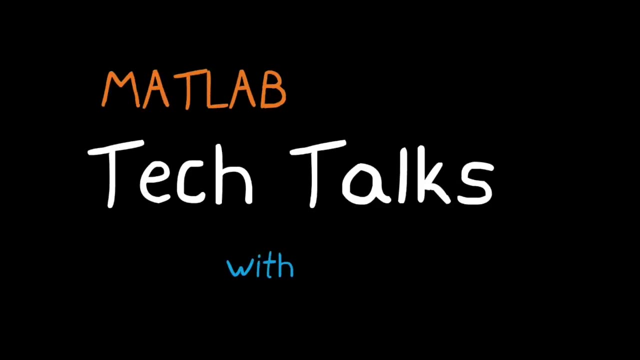 beneficial to talk generally about what it is that we're talking about today. So let's get started: How it works and why you might want to consider it for some of your projects. I hope you stick around for it. I'm Brian, and welcome to a MATLAB Tech Talk. As the name suggests, an adaptive. 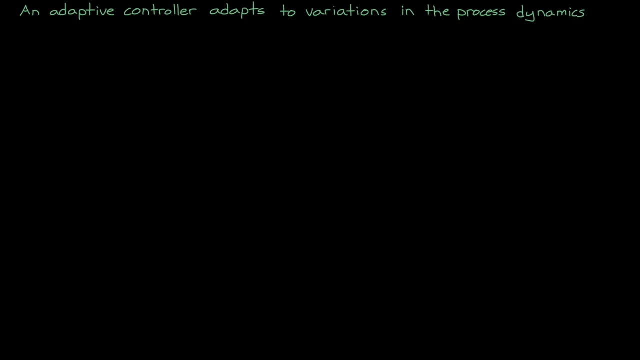 controller adapts to variations in the process dynamics, and these variations could come from a number of places. For instance, the disturbances that come from the environment might change, or, in some cases, variation just comes from the fact that you have uncertainty in your system. 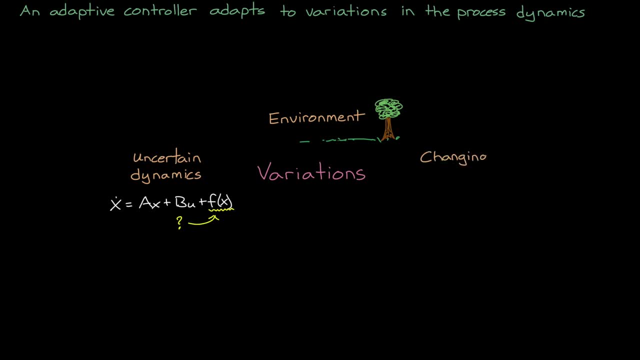 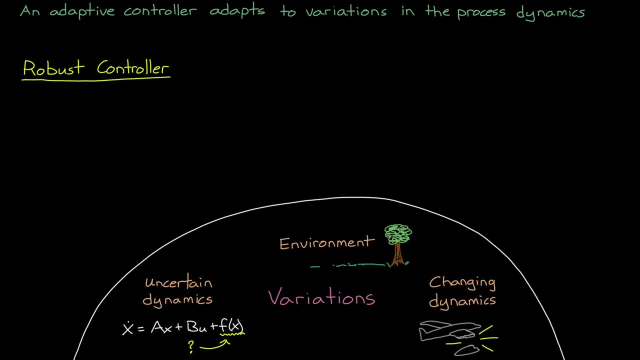 or unaccounted for dynamics in your model And finally, like in the case of the wing falling off, the system dynamics themselves might actually change, And a controller should be set up in a way that can handle these variations. One way to do this is with a robust controller. This means: 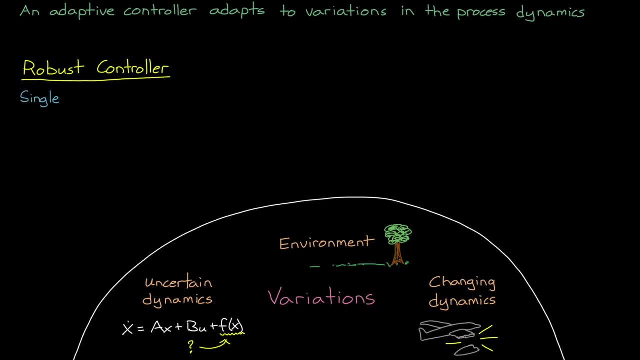 that the controller is designed with enough stability and performance margin that it works sufficiently well across the entire range of expected variations. And if a single static controller can do this, then it's a good idea to have a controller that can handle these variations, Then that's perfectly reasonable. However, finding a single robust controller that can 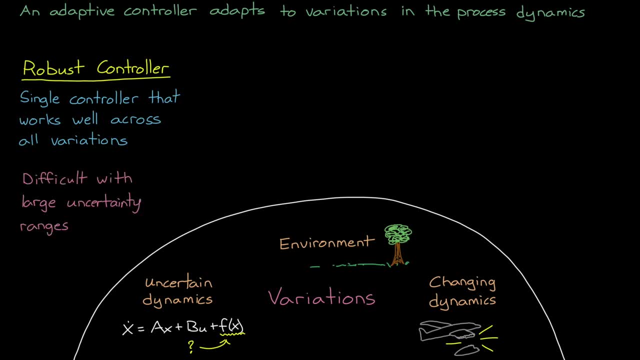 meet requirements becomes more difficult as the range of uncertainty grows. So for the cases with large variation, you may consider some other method, like gain scheduling that will change the gains of the controller as the system moves from one state to another. For example, you may 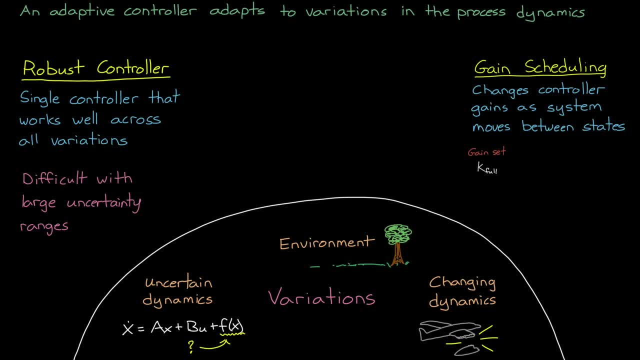 have a set of gains optimized for an aircraft with full fuel tanks and then a second set of gains which is optimized for near empty tanks, And then, through gain scheduling, the controller smoothly transitions between the gains as fuel is consumed, And this works well for variations. 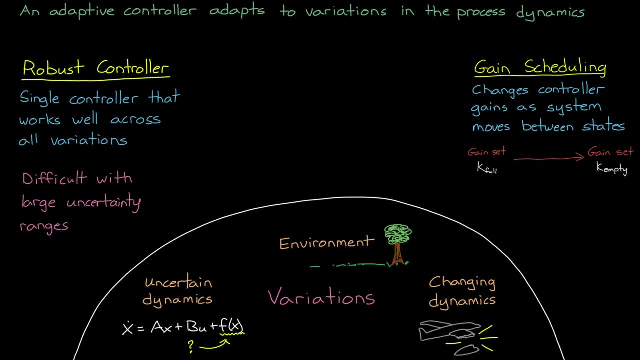 even large variations, but that you are expecting. It doesn't work too well for uncertain or unexpected variations, because you won't have already generated an ideal set of gains for them. So in the cases where variations are large and uncertain, it makes sense to do something else. 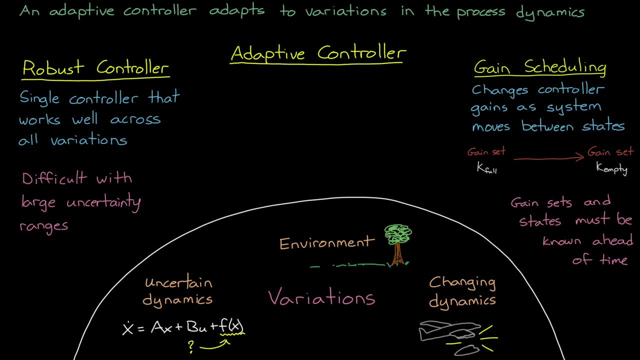 The gains or parameters of the controller are not completely determined ahead of time. Instead, a learning mechanism is built into the controller that is constantly tweaking and optimizing the parameters. Therefore, even if the controller encounters a situation that it isn't designed specifically for, it can still adapt to that situation by changing the parameters of 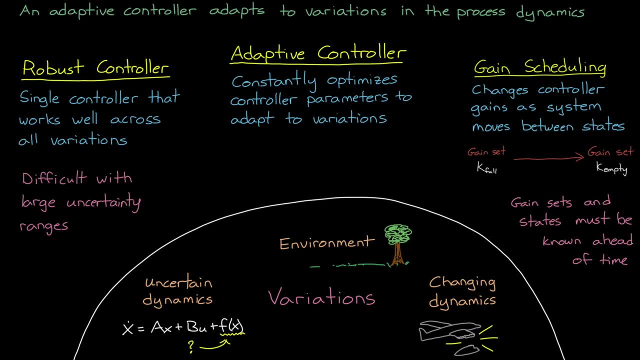 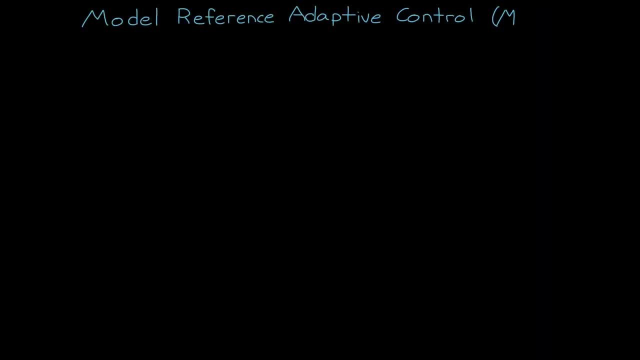 the controller in real time. So, with that being said, I want to go into more detail about one particular type of gain that can be used to change the parameters of the controller. If you're looking at a particular type of adaptive controller called Model Reference Adaptive Control, or MRAC, 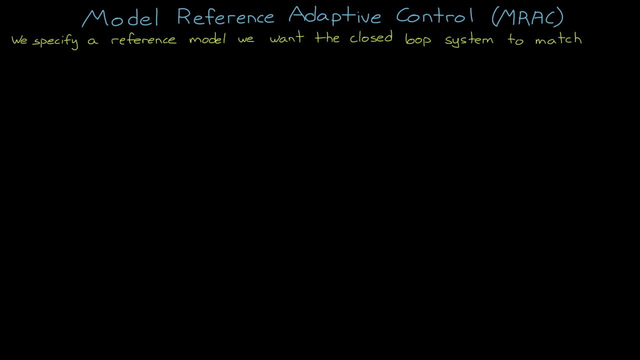 With MRAC, we specify a reference model that we want the closed-loop system to match. Let me try to explain it this way: Let's assume we have this real plant that we've modeled. with this state equation. We can manipulate this system through the control input u and then the system. 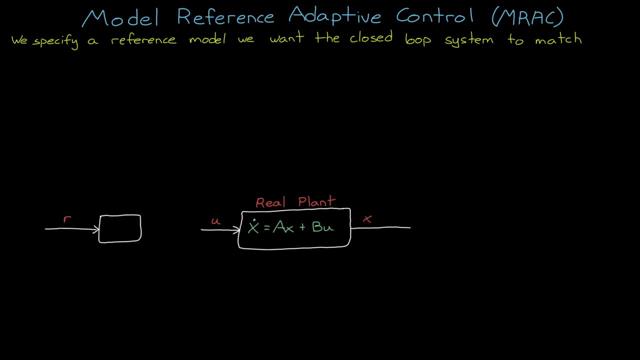 state x changes. And let's say we design a full-state feedback controller that can track a reference signal r. We have the reference input u and then the reference state x. We have the feedback gain kx and key forward gain kr. The idea is that we want to tune these. 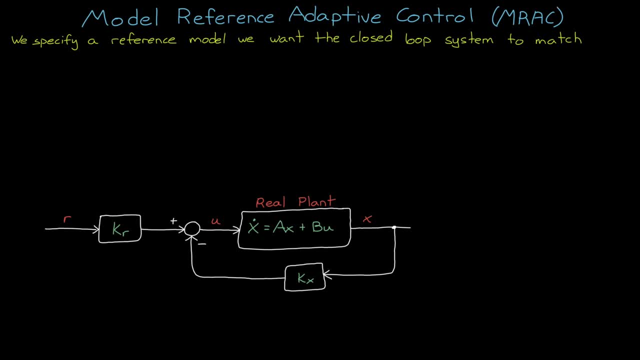 gains to generate the performance line we're looking for in this closed-loop system. Now, what performance are we looking for? Well, we could define performance in terms of things like Rise-Time and Overshoot and settling-time. However, alternatively, we can: 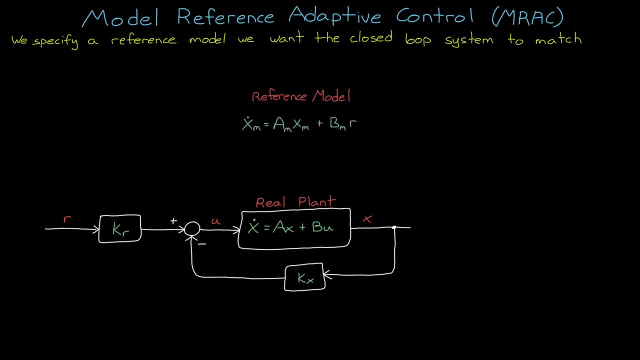 want to get this closed-loop system to behave like the Open-loop system, This other system we get to choose and it's our reference model. It represents the ideal behavior of the closed-loop system. So how can we ensure that these two systems match? Well, let's just take the simple approach where we solve for 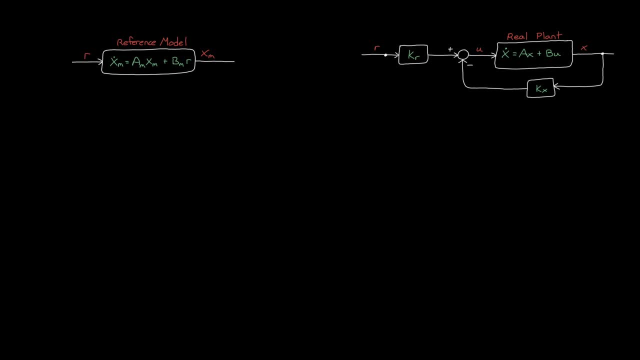 the state equations for both the reference model and the closed-loop system and then set them equal to each other. The reference model is just the state equation and to get the closed-loop system model we feedback the control input U, which is K R times R, minus K X times X. And now, by setting the 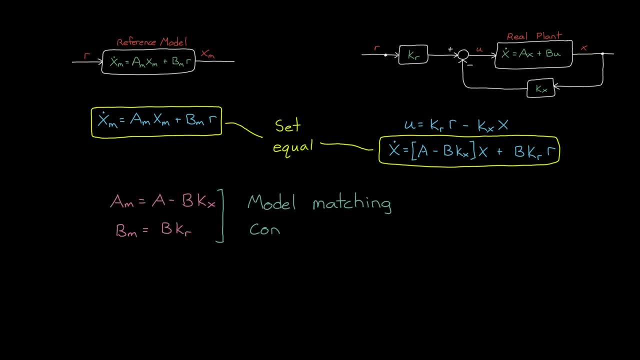 state and input matrices equal, we get the model matching conditions. Therefore, all we need to do is solve for K X and K R that make these two equations true. This is essentially pole placement, where we're choosing to place the poles of the closed-loop system at the poles of the reference model, But we don't necessarily 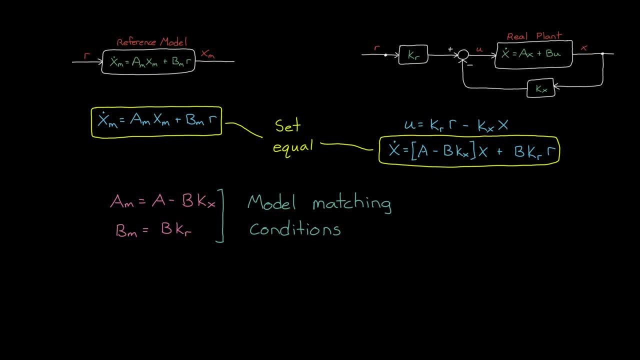 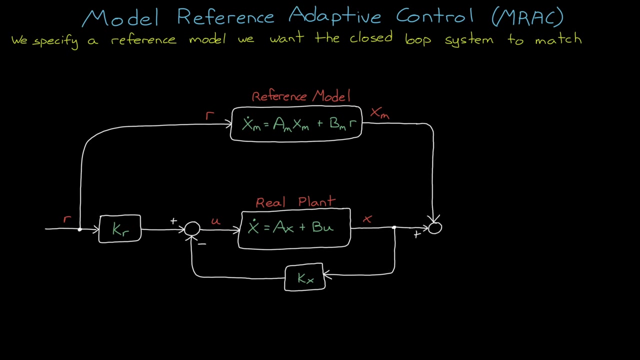 care about the location of the poles themselves. What we want is to have the state of the closed-loop system match the state of the reference model, That is, given the same reference signal, we want the outputs to match. So let's try this. We can subtract the two outputs from each other to. 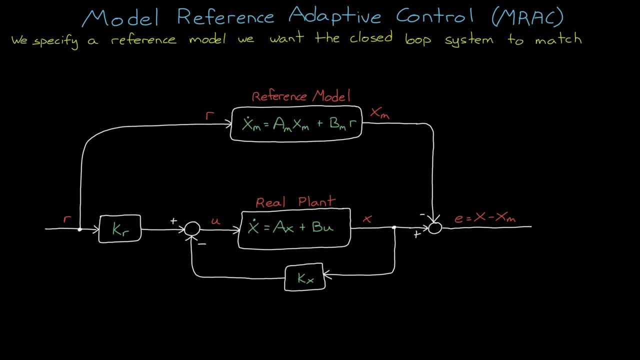 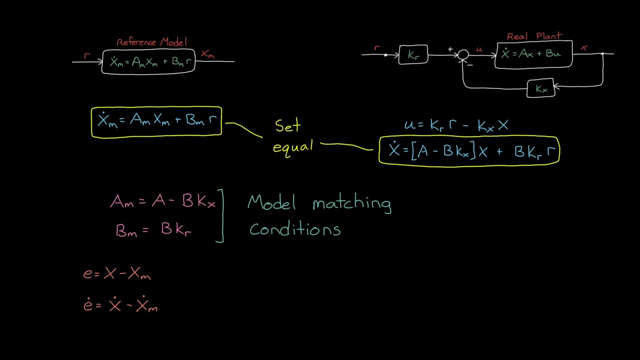 produce an error signal E, and the goal is that we ultimately want this error to go to zero, since that would ensure that the two systems have similar behavior for a given reference signal. So we have E equals X minus X M, and if we take the derivative of that, we get E dot equals X. 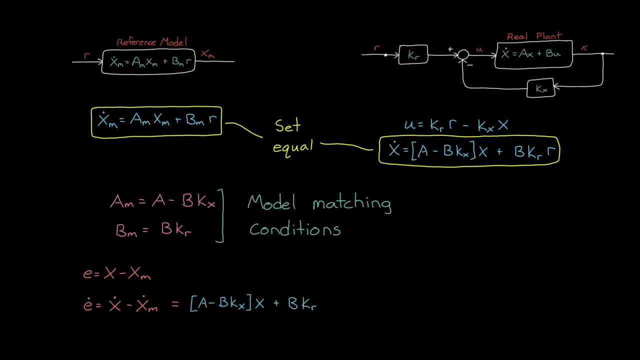 dot minus X, M dot, And after we substitute in the two state equations, we get this: If we now pick K X and K R that make the model matching conditions true, then these two terms will cancel out and this bit becomes AM and what we're left. 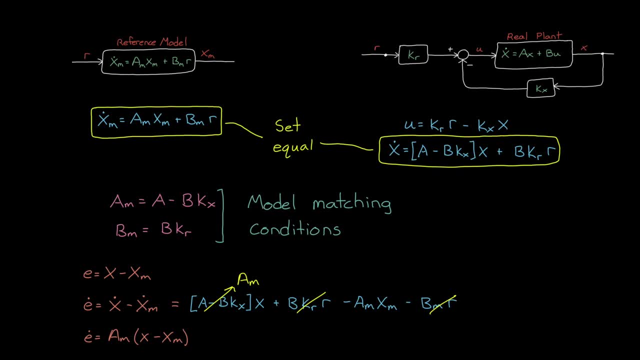 with is E dot equals AM times X minus X M, Or E dot equals X minus X M. Now, if you choose a reference model that is stable, that is, the real parts of the eigenvalues of AM are all less than zero, then this is a stable linear equation. 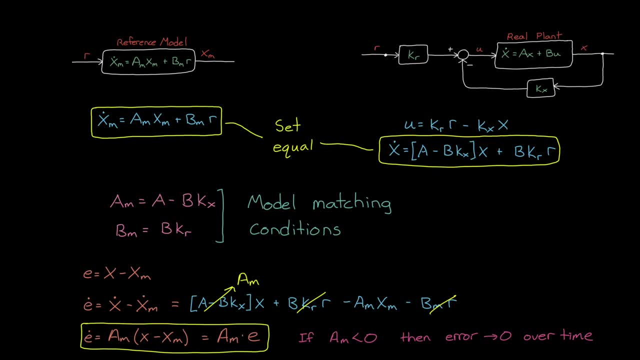 and the error will tend towards zero over time. So that means that even if we initialize these two systems with different starting conditions, as long as the model matching condition is met, the error will eventually go to zero and the outputs will be the same. And that's pretty cool. 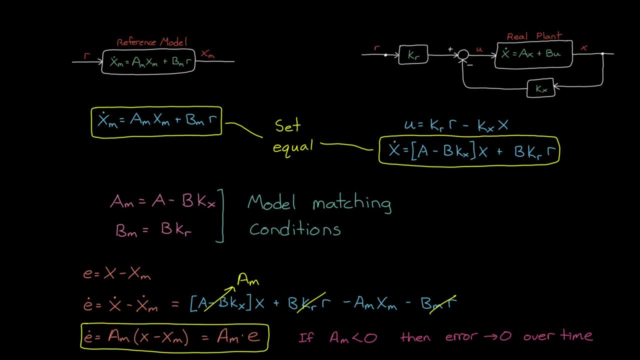 But you can probably see a problem with this in that it assumes that we have perfect knowledge of the system we're trying to control. That is, not only do we know the parameters A and B, but we also know that the model itself perfectly captures the dynamics of the real system, Which, if we knew that, we wouldn't need. 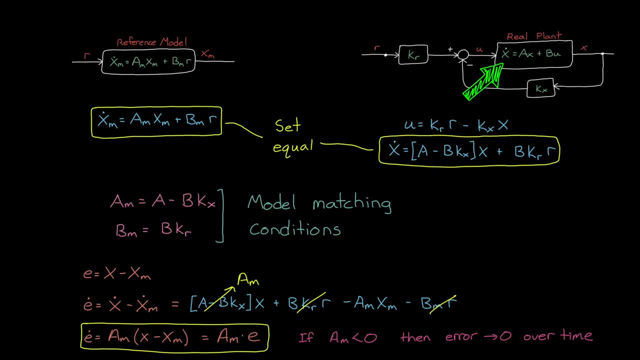 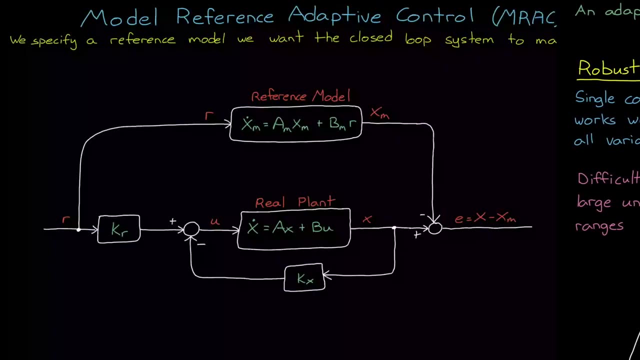 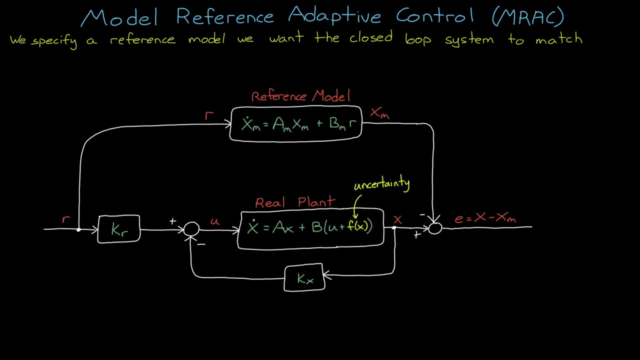 adaptive control in the first place. But we know that isn't the case because we already talked about all of the uncertainty regarding the variations in the system. So there's going to be some amount of uncertainty. F of X, That makes picking KR and KX. that's going to perfectly match. 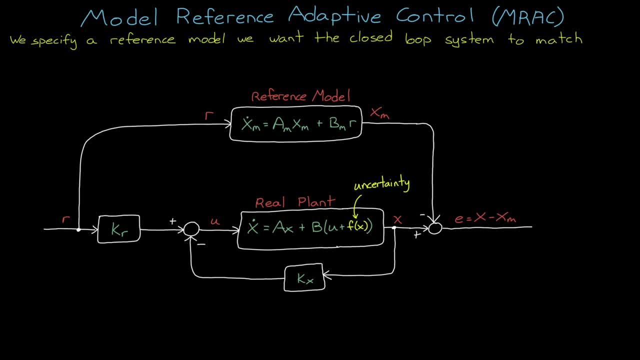 the closed-loop system to the reference model impossible. We are out of luck, Except maybe we aren't, because we can try to do something about it. If we can cancel out that uncertainty, then we'll be left once again with our nominal model, and our model matching conditions will still hold. So to cancel F of X we 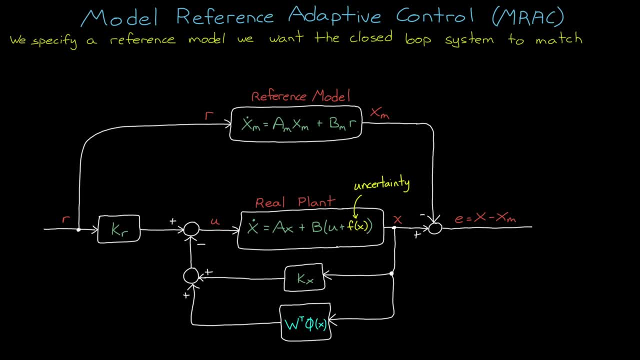 can feed back another term, W transpose times phi, Where W is a vector of adaptive control weights and phi is a set of uncertainty model features, And I'm going to explain what that means in just a bit, But for now, if W transpose times phi perfectly matches F of X, then these two terms will: 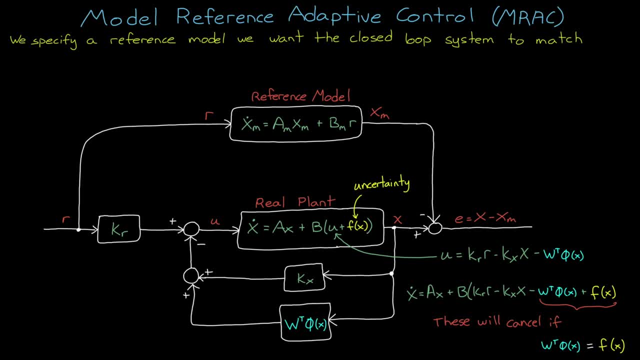 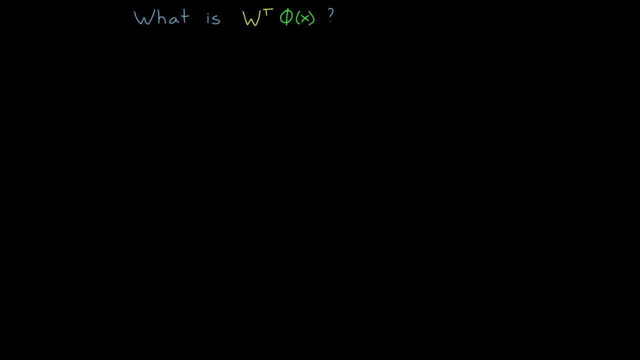 cancel out and we'll just be left with the nominal model of the system. Alright, so that's our new goal. We want to match W transpose phi to the unknown F of X. So what is W transpose times phi? Well, it can sort of be anything you want. 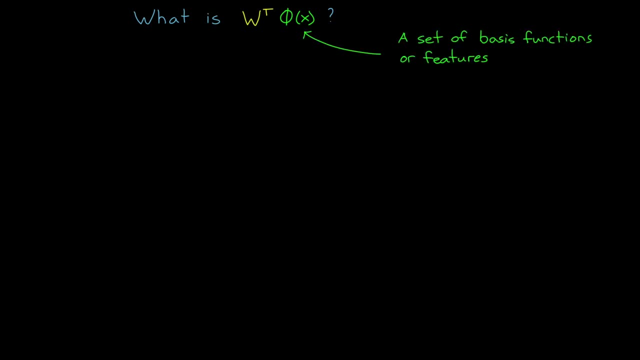 Phi is a set of basis functions or features that you can choose, which can then be combined using the weighting vector W. For example, let's assume a system has two states, P and theta, and that the unknown variations to the system are: F of X equals 1 plus 3 times theta plus 2P plus the absolute value of. 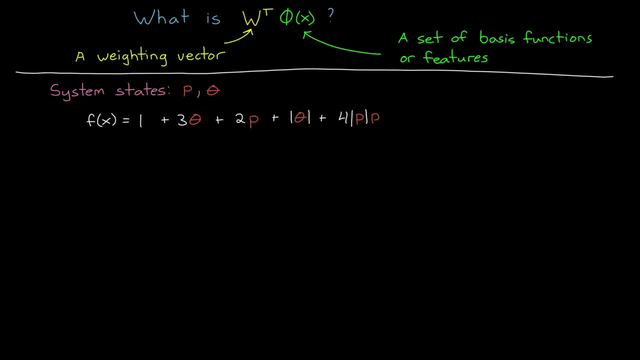 theta 4 times the absolute value of p times p plus theta cubed. In this case, an absolute ideal phi would consist of a bias 1, plus the other features, theta p, the absolute value of theta, the absolute value of p times p and theta cubed, And then the absolute ideal weights would be 1,. 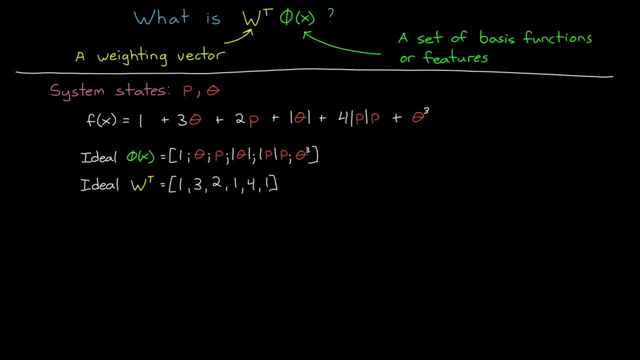 3,, 2,, 1,, 4, and 1.. And the combination of these two would perfectly represent the unknown variations. and if you knew all of this, then you could set up w and phi accordingly. However, more often than not, we don't know what the model of f of x looks like, So we don't know what the 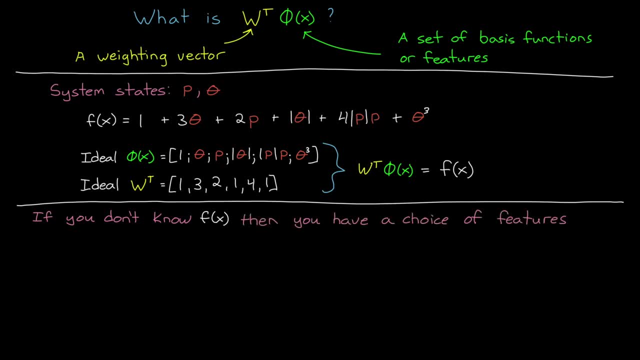 ideal features are and therefore we have to make a choice as to which features we want to use. We could simply choose to model phi as the ideal model of f of x, and then we could set up w and phi as the ideal model of f of x. 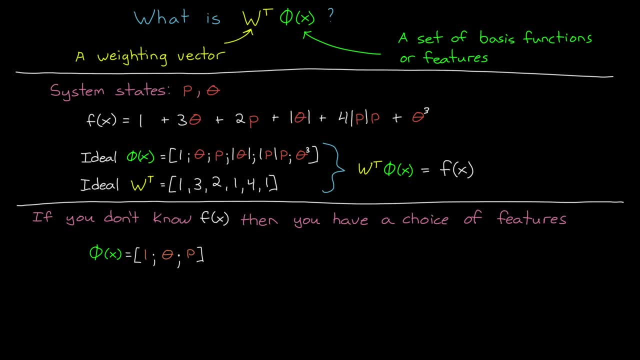 states of the system plus a bias, And then, in this case, we'd essentially be making a linear approximation of this nonlinear function, And that's still better than nothing, but it won't be perfect. However, if we had some understanding of the structure of the variations, like 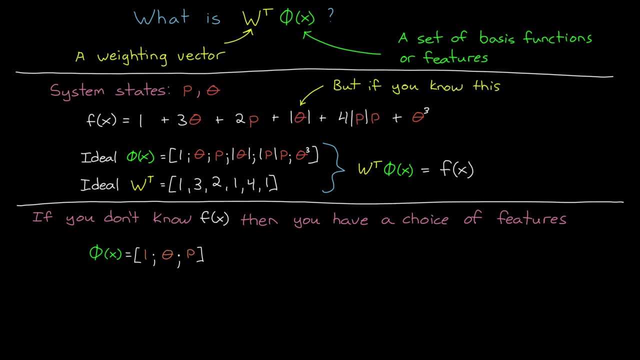 for example, we know that there's a term that is proportional to the absolute value of theta, then we could add that additional term to phi, and now our approximation would include at least one nonlinear term and the fit will be better. However, 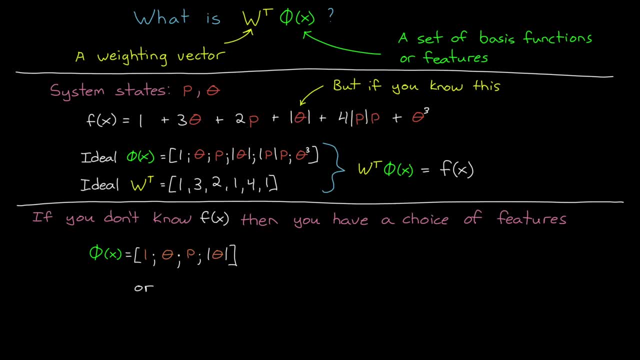 if you don't know much about the individual features of f of x at all. it's common to use a set of general features like radial basis functions that are universal approximators. This just means that you can represent any arbitrary function f of x as long as you have. 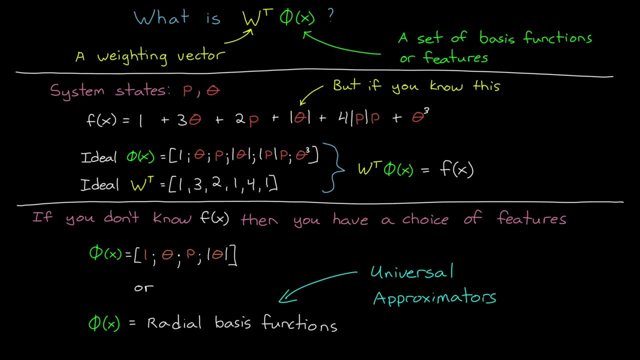 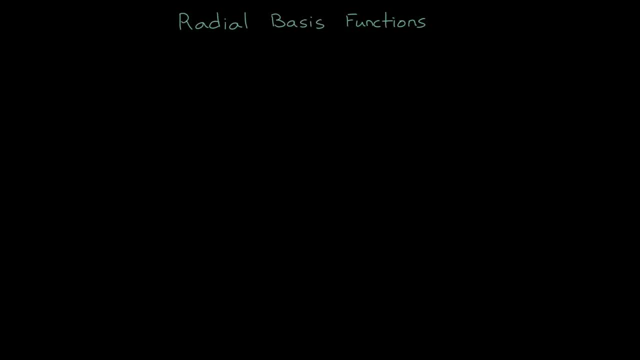 enough of them and set them up correctly. Let's look at radial basis functions a little bit more so that you know how they work. There are several different shape radial basis functions, but for this example, we're going to focus on a Gaussian shape. Therefore, a radial basis function is: 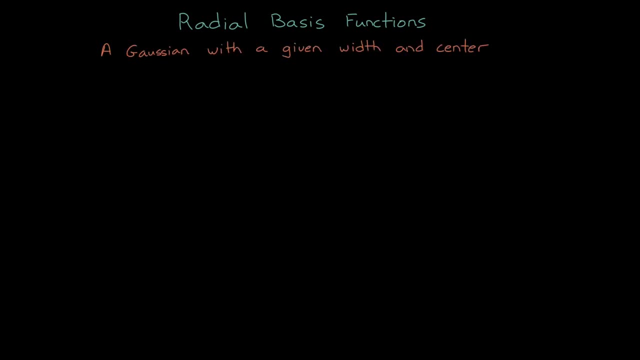 essentially a Gaussian that has a given width and center, And if we have multiple Gaussian functions, we can build up a function approximation by scaling each one by a different weight and then summing them together. For example, here I have a Gaussian that I can scale with a weighting factor. 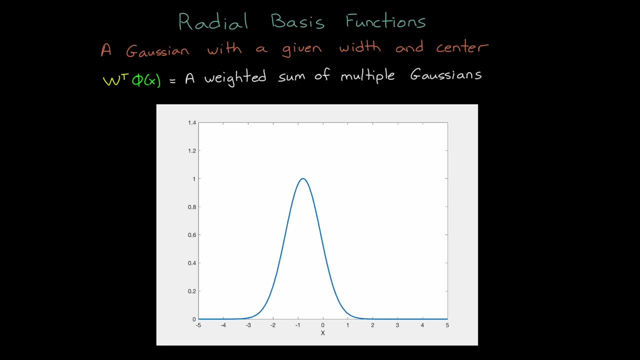 I can adjust the width of the Gaussian and I can move the center. Now I can add two more Gaussians, centered at minus three, and three each with the same width, And they all currently have the same height as well, or a weighting factor of one. Now the product of W, transpose and phi is 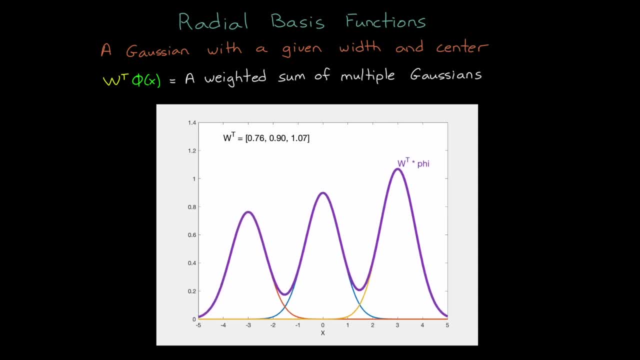 the function approximation, And by adjusting the weights or the height of the Gaussian we can affect the shape of that function, And the idea would be to find a set of weights that produce a close estimate of the uncertainty f of x. However, there's not much flexibility if we just use three radial basis functions, So we may want to. 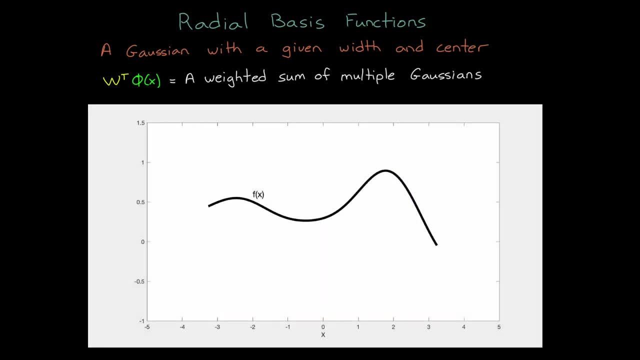 increase the number. For example, let's say that this black line is the real uncertainty function f of x. Now we define 20 radial basis functions that span across the input space And I've initialized W to be point three for each Gaussian. And the purple line is the result of W transpose. 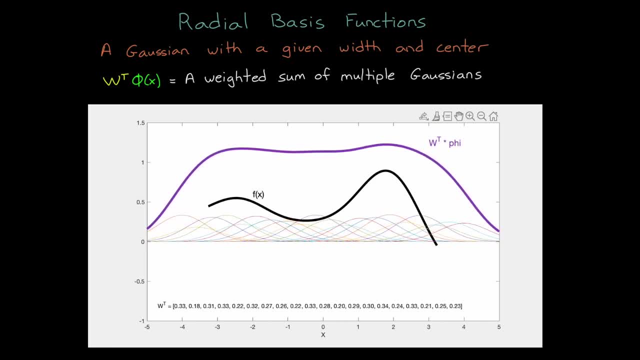 times phi. And at this point we can start adjusting the weight vector, which changes the amplitudes of each of the Gaussians, Which then changes the estimated function until we get to some optimal set of weights. And finding this optimal weight vector is where adaptive methods come into play. If you have a nominal 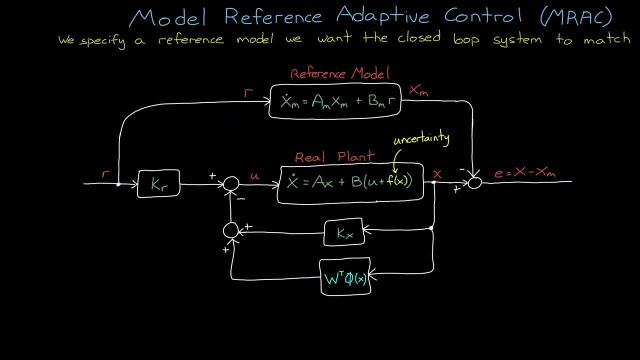 model and a reference model and a set of basis functions defined. then you can use them, along with the error term and the reference signal, to learn W over time. In this way, we're converging into a set of basis functions that can cancel them out, But we can actually do more than just. 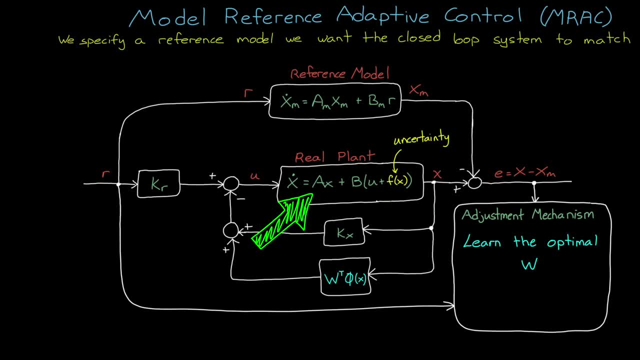 learn the unmodeled dynamics, Because if you don't have a nominal model at all and therefore no way to come up with a nominal Kr and Kx, we can also set up the adjustment mechanism to learn Kr and Kx. So at the exact same time, we can learn the unmodeled dynamics, so we can cancel them out. 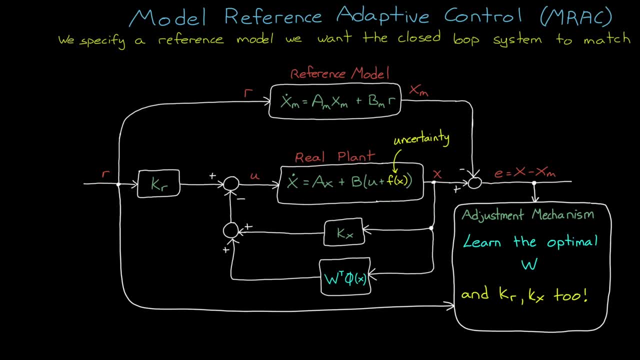 and learn the control parameters to reach that model matching condition. And at this point we'll see how well these algorithms do that And unfortunately the math would take a video on its own to describe. But fortunately other people have already created those videos. So if you want, 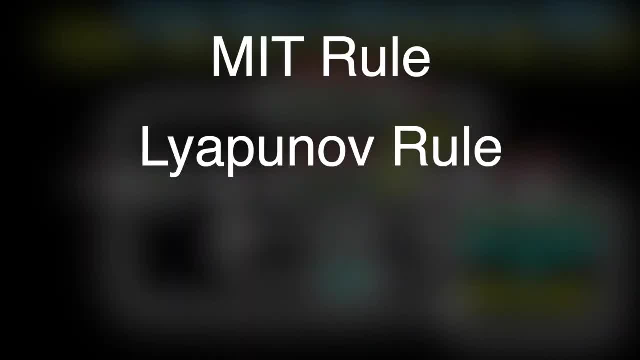 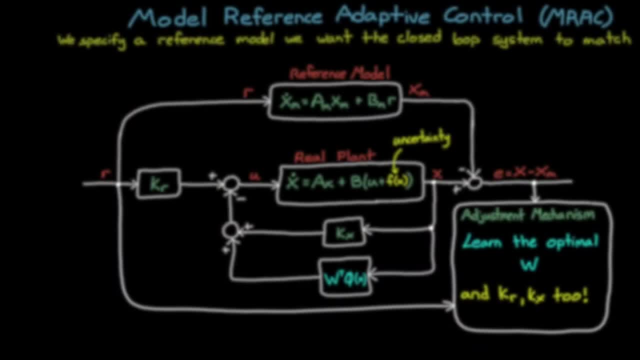 to learn about the MIT rule or the Lyapunov rule. for learning these parameters, I suggest you check out the great resources that I've listed in the description of this video And hopefully, with this brief overview of the control law and the block diagram, you'll have a better appreciation. 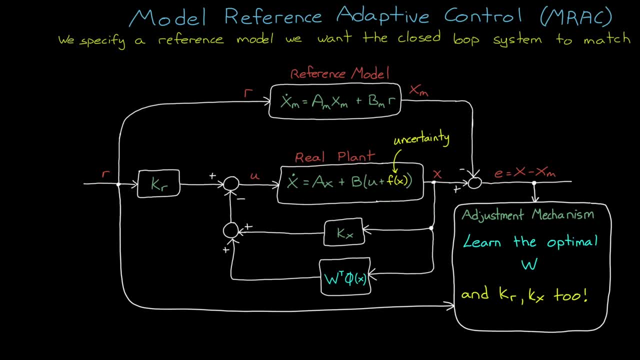 for what MRAC is trying to do, And that'll make going through the math a little bit easier. Now, before I end this video, I want to show you a version of model reference adaptive control in action. This example shows how to use MRAC to 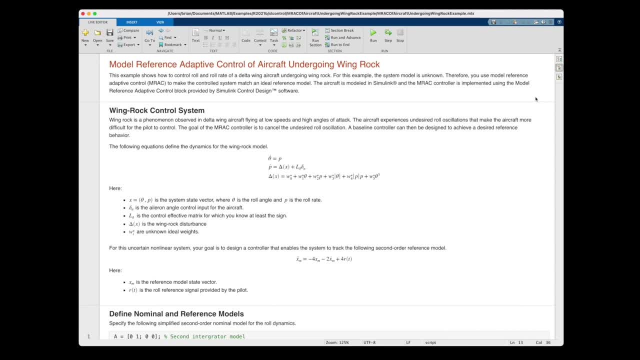 control the roll of a delta wing aircraft by canceling out the undesired roll oscillations that can occur, And it uses the model reference adaptive control block in the Simulink control design software. The general problem is that with delta wing aircraft that are flying at high angles, 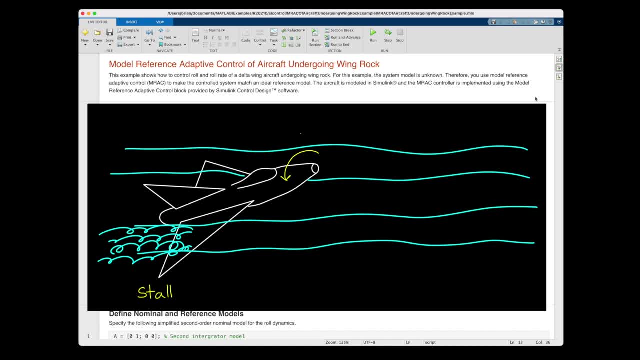 of attack. the stalling of one wing before the other can induce a roll and a slight turn that will stop the stall on that side but then cause the other wing to stall, And then the opposite happens, causing a back and forth oscillation, And high angles of attack are seen when the airplane. 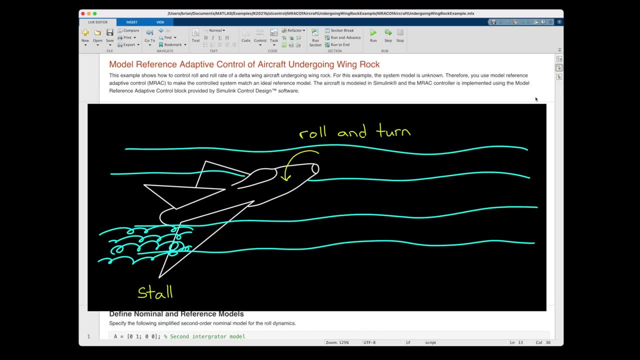 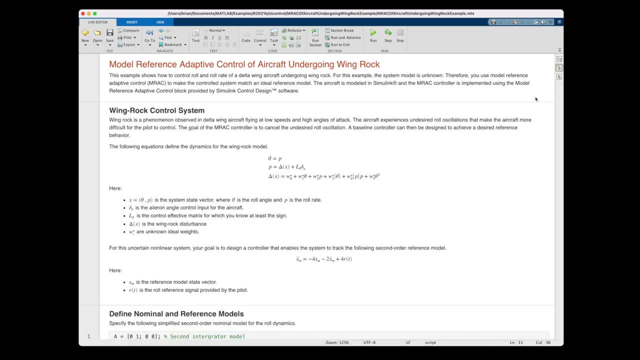 is landing, which is not an ideal time to kick up these disturbances. So let's see how this example uses MRAC to learn these disturbances and cancel them out by moving the ailerons. So this is the MRAC control model and it's saying that the roll rate is the derivative of roll angle. 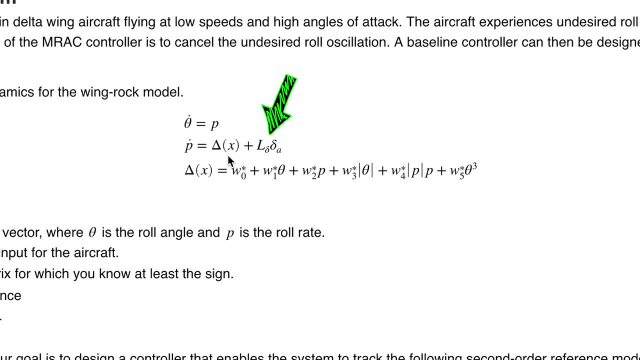 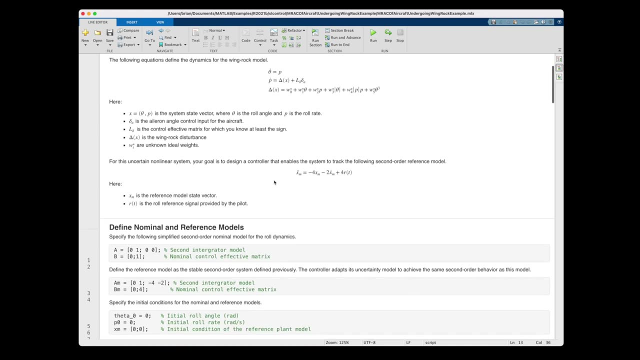 and the angular acceleration is affected by the angle of the ailerons, plus the unknown roll dynamics, delta x caused by the stalling wings. This is the f of x that we won't have modeled but are hoping that the MRAC controller can estimate and cancel out. And down here we define. 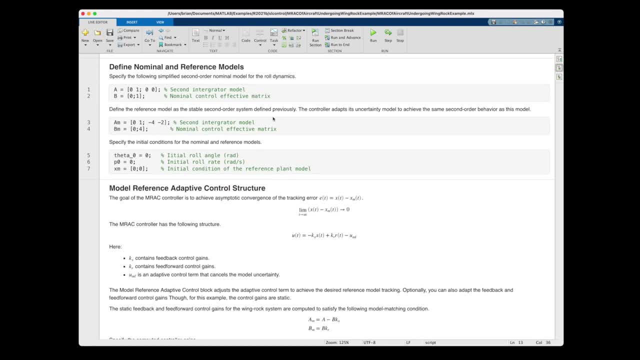 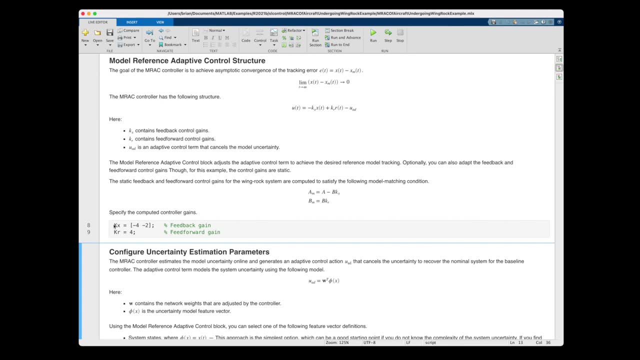 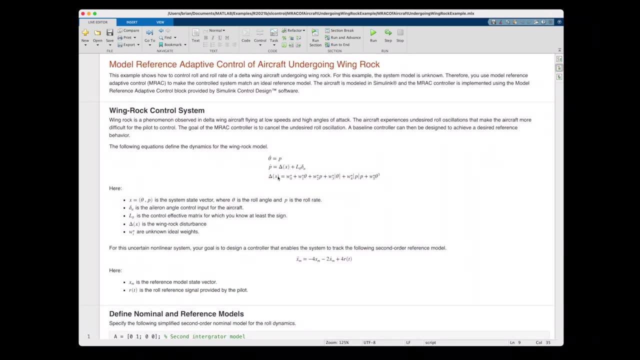 the nominal model of the aircraft and the reference model that we want the closed loop system to behave in, So we can use the model matching conditions to specify a kx and kr. Now we need to specify phi Again. if we knew the structure was in this form up here, then we could just use those features. 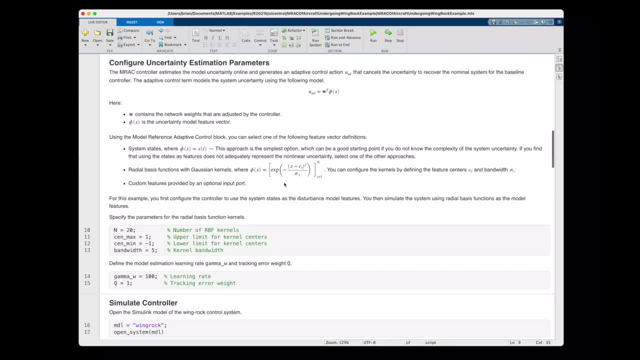 directly in phi. However, since we don't, this example opts to use system state as the feature set at first, and then 20 radial basis functions afterwards, so that you can compare the performance of both. Now we can simulate the performance of the controller in Simulink. 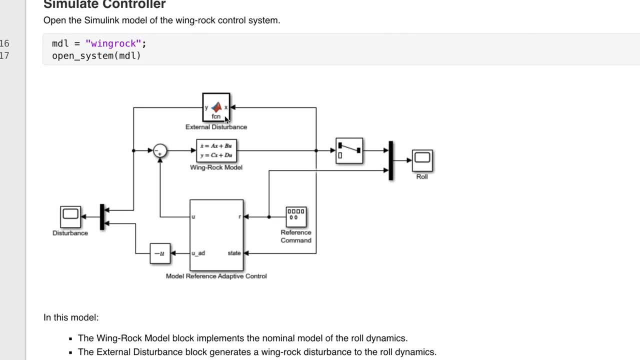 Here we have the true airplane model and the true external disturbances. And then this block is the model reference adaptive controller that's taking in the reference command in the current state of the system and then, using an adaptive mechanism, it's learning the parameters of w in order to 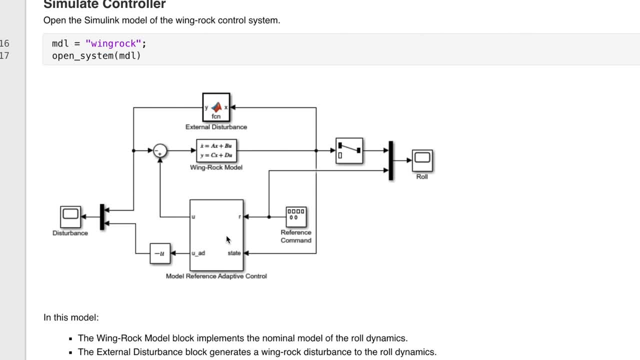 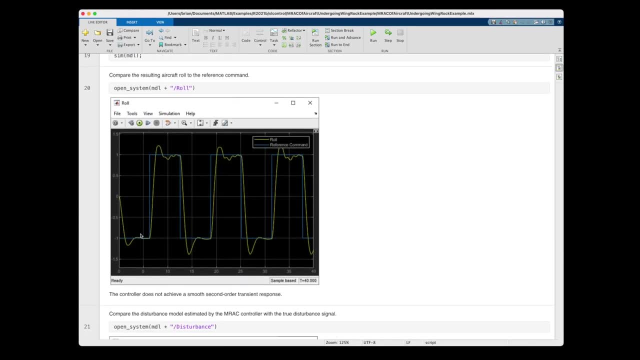 cancel out the disturbance And then this block outputs the control signal u and the estimated disturbance. And if we scroll down you can see the role tracking capabilities of this controller when we use phi defined as system state. And we can see the control signal u defined as system state.